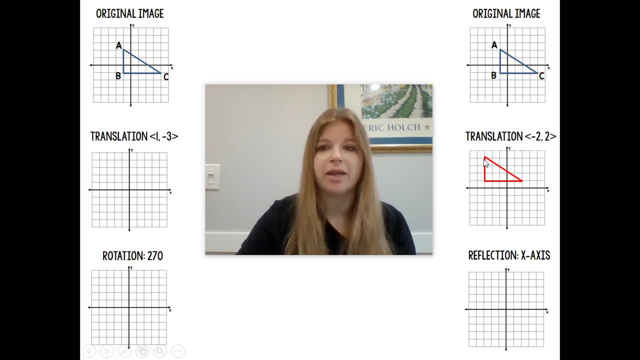 units up, it would be in this point of negative 3,, 4.. And then everything else would go in that same Translation pattern, And you can see exactly where those points would be Now if I was to take that new figure, that new image, and have it undergo a reflection in the x-axis. So what that means is I: have to take that triangle, reflect it over the x-axis, have it flip right over, which would mean this: A prime is going to become A double prime over here in the third quadrant. So if A prime is at negative 3,, 4, and I reflect it over my new image. 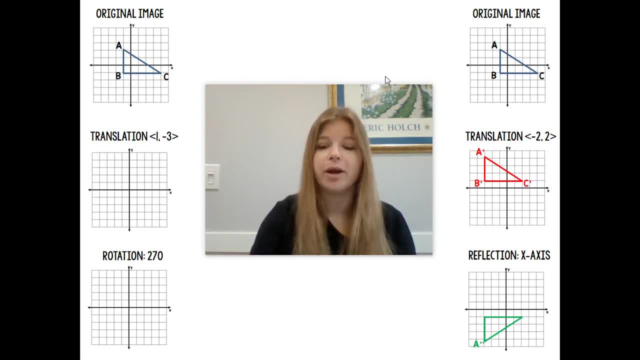 A prime would be at negative 3,, negative 4, and so on: B prime and C prime. So if I was having this original image here, undergo a translation of negative 2,, 2, and then a reflection in the x-axis, this would be my final result. Notice, my image gets my primes. 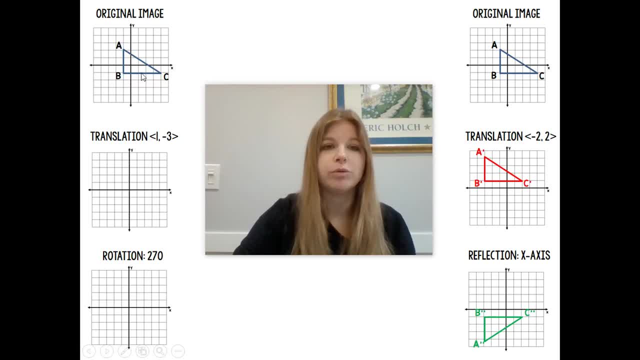 Notice: the next image gets double primes. Same thing here. Original image ABC. it's the same triangle as the previous one. If I had this triangle undergo a translation of 1, one negative three, One negative three means I'm going to go to the right. I'm thinking about your. 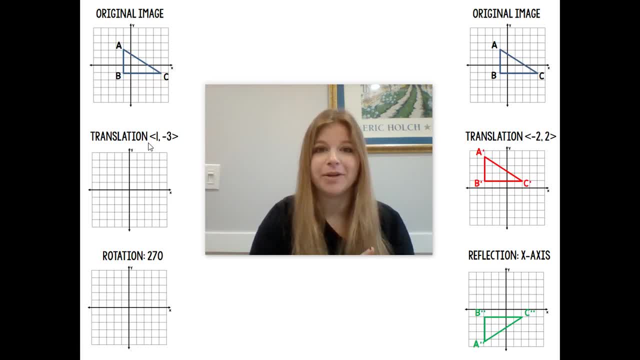 right To the right one and then down three units. So if I took this figure and turned to the right one and then down three units, my figure would be here along with A prime, B prime, C prime. Okay, Then if I wanted to rotate this figure 270 degrees- remember rotating a figure 270 degrees? 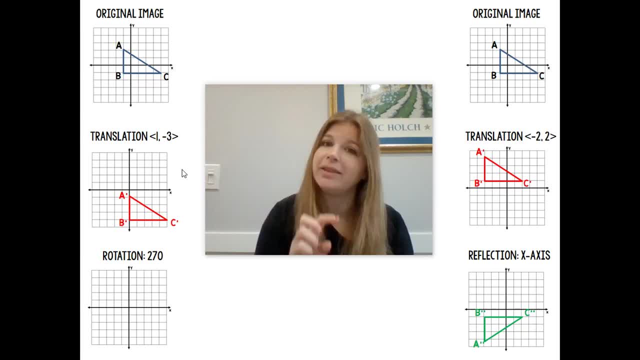 would be like it, rotating 90 degrees in 180 or 180 and then a 90. But coordinate wise, it's Y negative X. So if I was to look at each one of these new ordered pairs for my A prime, B prime, 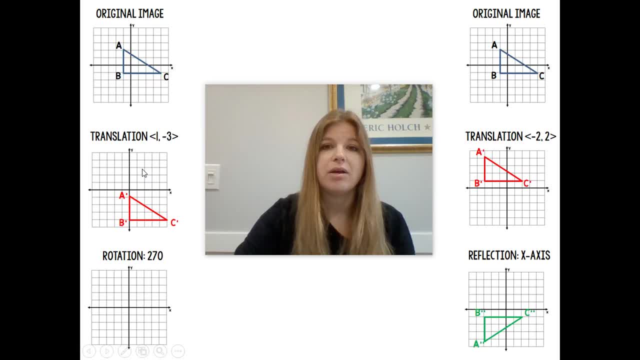 and C prime and then put my new points as Y negative X. it would rotate it from the fourth quadrant through the first, Second and then into the third. It actually is going to be here in this form, Okay, So if I was, 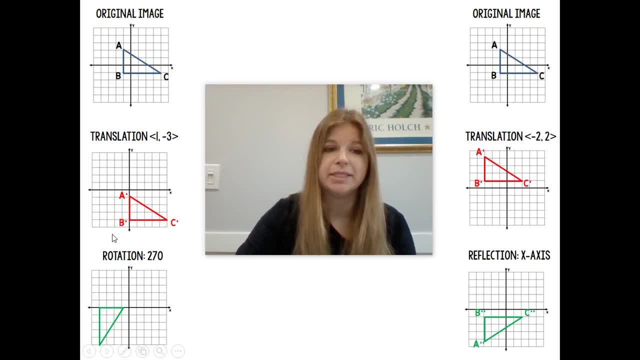 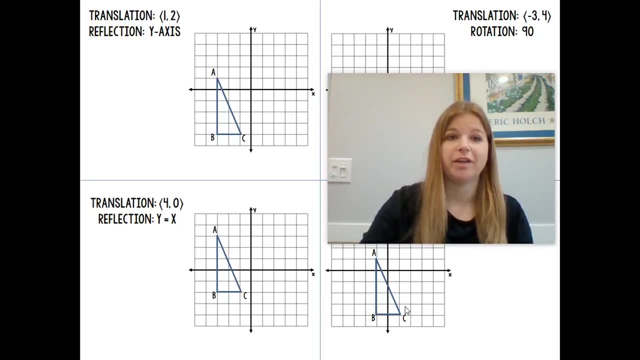 to take this figure and rotate it 270 degrees, my A double prime, my B double prime and my C double prime would end up being in this: Okay, So now we've got this new figure, ABC, this triangle, and we're going to do the composition of these two transformations. We're going to translate it. 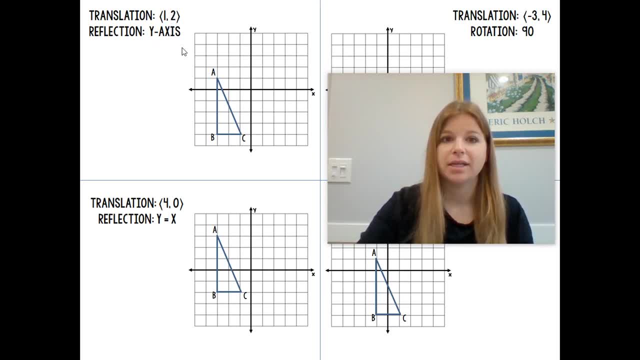 one, two and then do a reflection in the Y axis. So what we're going to do is we're going to do a reflection in the Y axis. So what we need to know from our previous problems that we did before, if it has this translation of one, two, what does that mean to do? 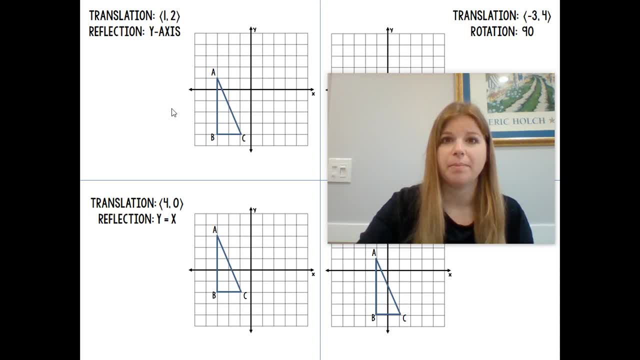 That would mean to move it one unit to the right and then two units up. So if I did that transformation it would look like this: One unit to the right, two units up, And for every point it would be the same: One unit to the right, two units up, One unit to the right and two units up. 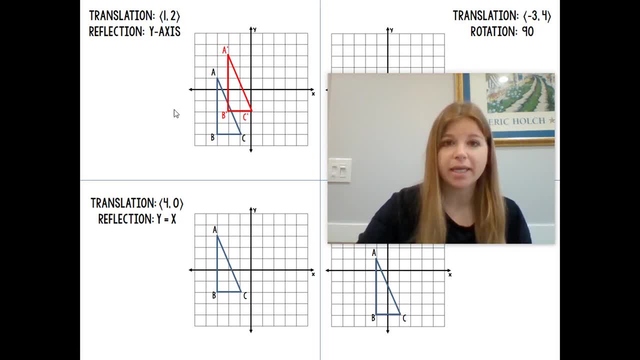 until I have my A prime, B prime, C prime. The second transformation that I'd be doing in this composition is a reflection over the Y axis. So here I have my Y axis. A transformation over the Y axis means that my Y coordinate stays the same. 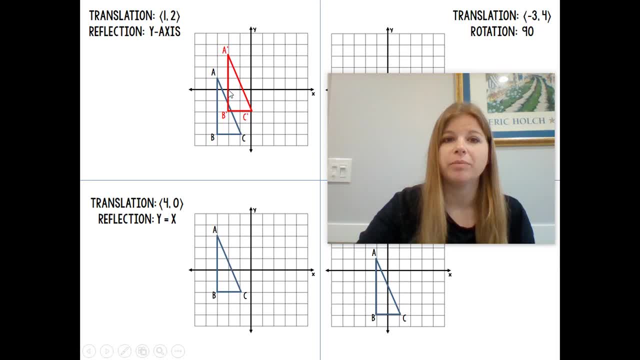 when my X value changes its sign. So from going from negative two positive three, I would then go to positive two positive three And my reflection would look like this: a reflection over that Y axis for A prime, B prime and C- I'm sorry, A double prime. 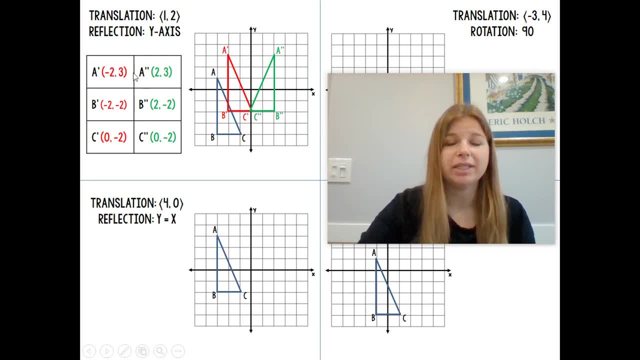 B double prime and C double prime. If I look at the table of values of these two figures that we just created, notice from the original figure of negative three, one I would be adding one, adding two, And that's where there's this: A prime, B prime, C prime would come from, If I'm reflecting over. 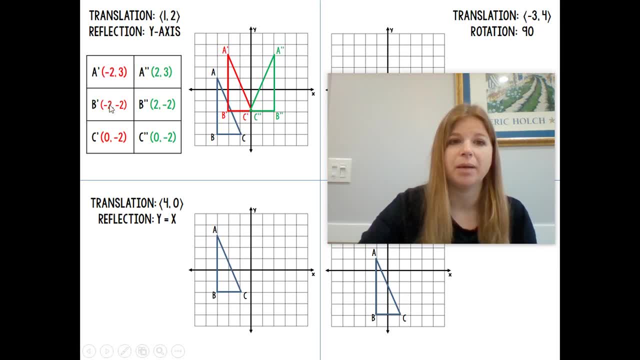 the Y axis, notice the change. The change then just simply becomes that the X values become its opposite sign. So negative two becomes positive two and negative two becomes positive two. Zero would just say zero. So I would be adding one, adding two, and that would be positive two. 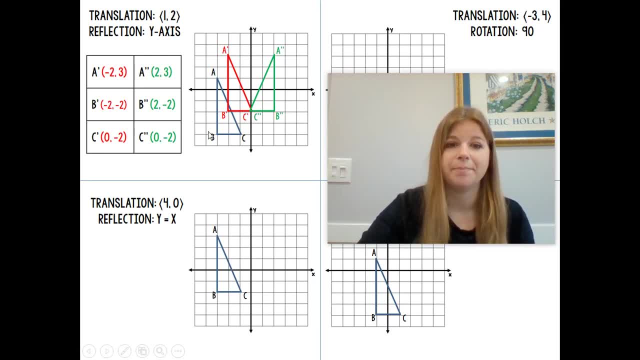 So I would be adding one, adding two, and that would be positive two. So I would be adding one and notice all the Y coordinates stay the same. Now we're going to take this new figure, translate it: four zero with a reflection over Y equals X. So a translation of four zero would: 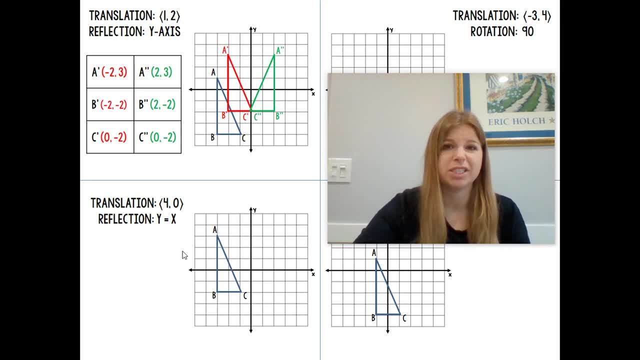 mean four units to the right and zero units up or down, So it just kind of stays there. It's just simply a horizontal change. So my new figure, after a translation of four zero, would be at this point: all points four units to the right. That's all. four zero would tell you to do. 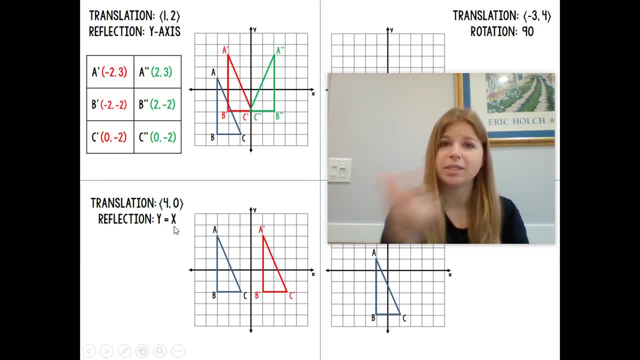 Now, a reflection of Y equals X would mean that my X and Y coordinates flip. They reverse each other, They switch spots. I don't change any signs or anything like that. So if A prime is at one three, then A double prime would be at three one. It would be right here. 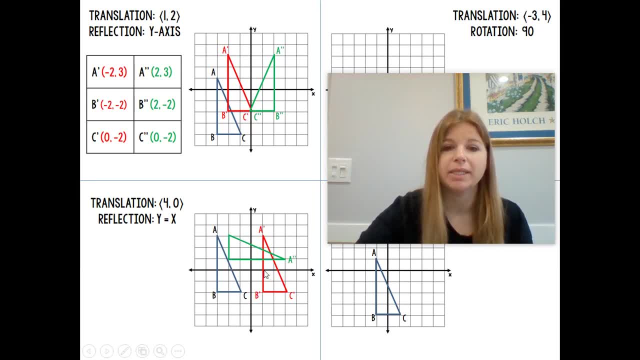 Okay, that's where A double prime would be. If B prime is at one negative two, then B double prime would be at negative two, one which is here. If C prime is at three negative two, then B double prime would be at negative two, one which is here. 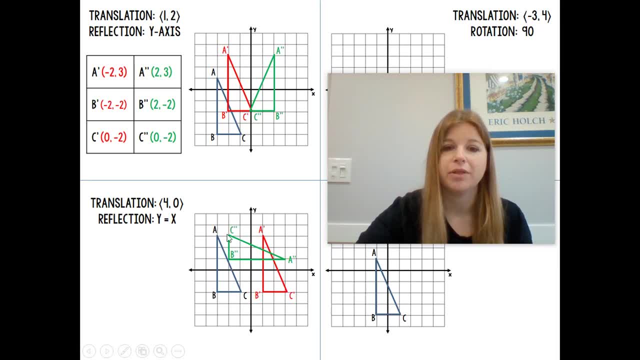 Then C double prime would be at negative two, three, And those are our points. So a translation of four zero would mean that I have to find these ordered pairs and add four to every X And then notice the reflection: Y equals X just means I'm simply switching the X and Y values. 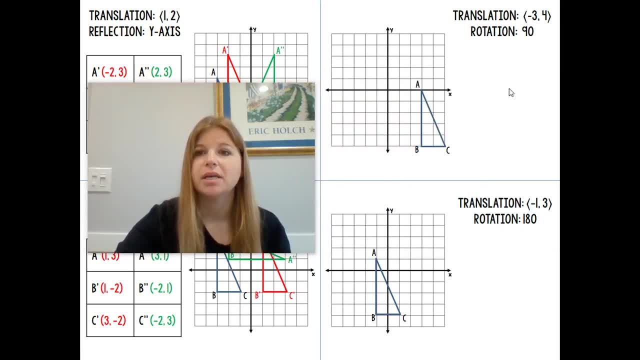 Now let's take a look at translations and then rotations. So a translation of negative three four would mean I take this point and move it three units to the left, and then I take this point and move it three units to the left. Now let's take a look at translations and then rotations. So a translation of negative three four would mean I take this point and move it three units to the left. 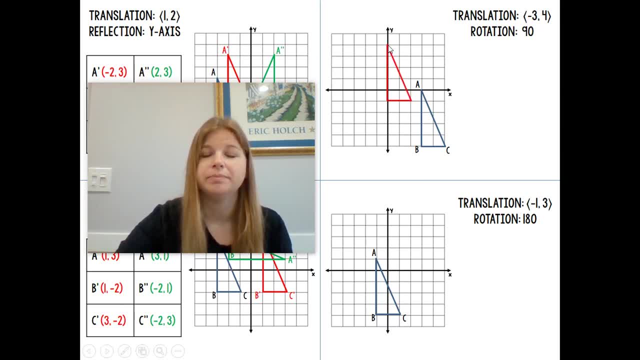 four units up. So this is where A prime should be: Okay: three units to the left, four units up. B prime: three units to the left, four units up. C prime. Now, a rotation of 90 degrees means I'm going to be taking this figure and I'm going to be rotating it this way. 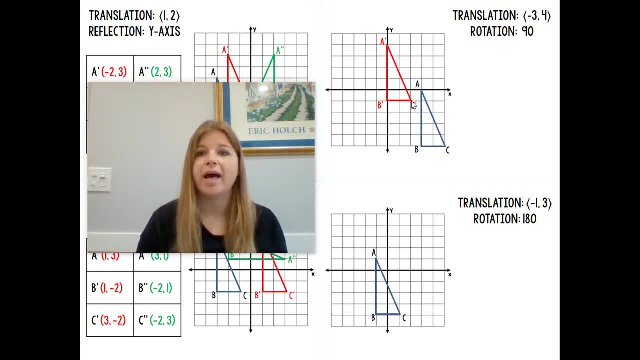 Okay, it's going to go to the left. So that triangle that you see is mostly in quadrant one is about to get put into mostly quadrant two. If I also take a look at this point here of zero four, at A prime the rotation of 90 degrees would be negative four, zero. 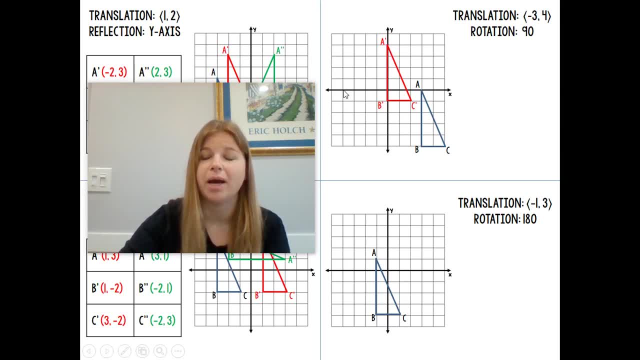 I'm switching the X and Y value and I'm making my, my Y value here become my X negative. So it's negative Y, X, A prime, A double prime would be here, B prime at zero, negative, one would become one zero. So I change the sign of the Y to become my X and I keep the Y value. 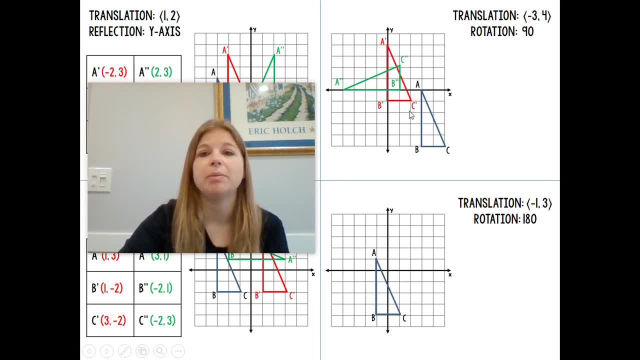 I'm sorry, the X value is my Y And then C. double prime would be in this point here. So going from negative three, four- translation three units to the left, four units up and then rotating at 90. And again you can see it becomes negative Y, X, negative Y X, negative Y, X.